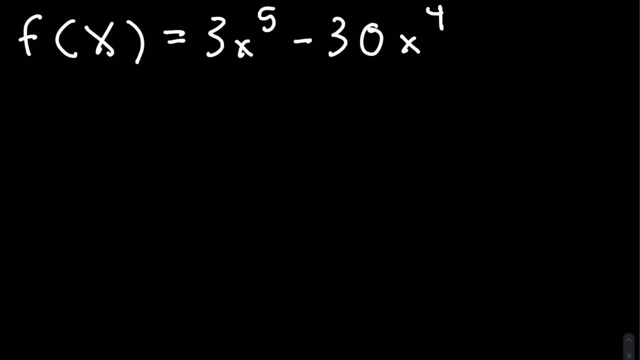 point of inflection. So let's try an example. Here we have the function f of x is equal to 3x to the fifth minus 30x to the fourth. So let's try and find out if there are any inflection points and what they are if they do exist. So the first step when finding inflection points 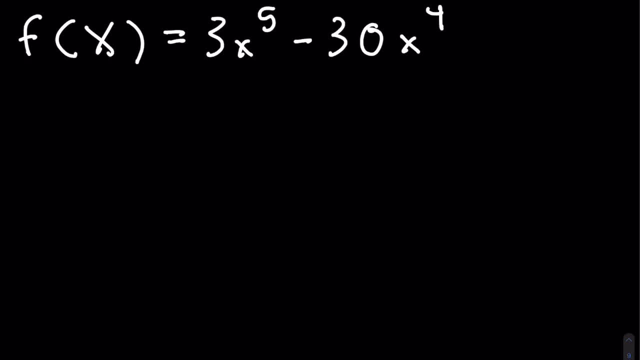 is to find the second derivative of your function. So let's go ahead and do that. So the first derivative of our function is 3x to the fifth. So we take the derivative of that, we get 15x to the fourth, And then we take the derivative of. 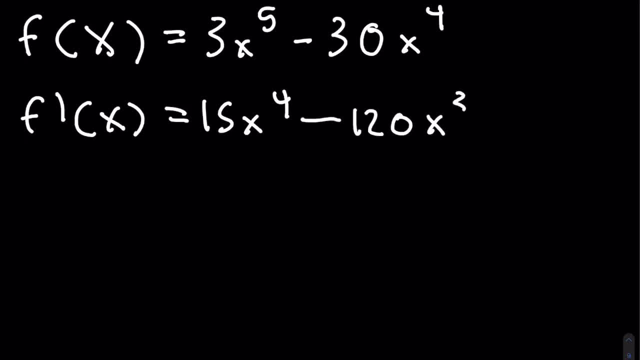 30x to the fourth, which is 120x cubed. So now we need to get the second derivative, So we need to take the derivative of this. So the derivative of 15x to the fourth is 60x cubed. 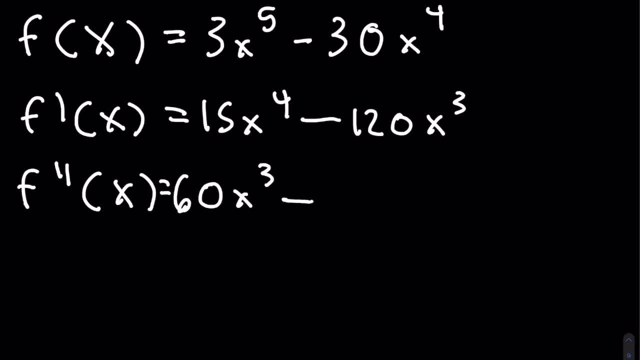 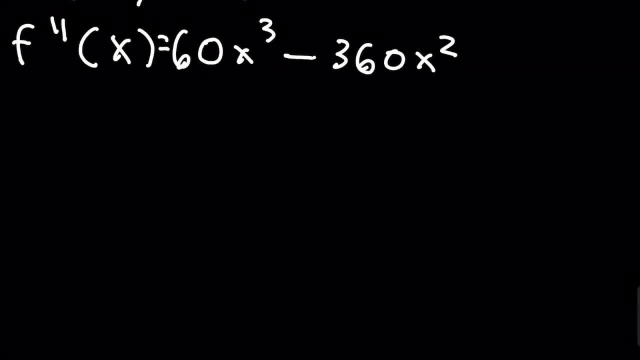 And then we need to take the derivative of minus 120x cubed, which is 360x squared. So after you find your second derivative, what you want to do is take your second derivative, set it equal to zero and then solve for x. So let's go ahead and do that. So we have 60x. 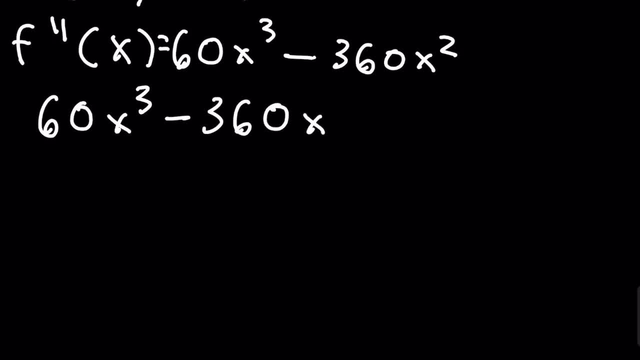 cubed minus 360x squared equals zero. So when we solve for x, what we want to do is try and factor something out of this. So what could we factor out of this? We could factor out a 60x squared. So if we factor out a 60x squared from 60x cubed, we'll just get x And then minus. 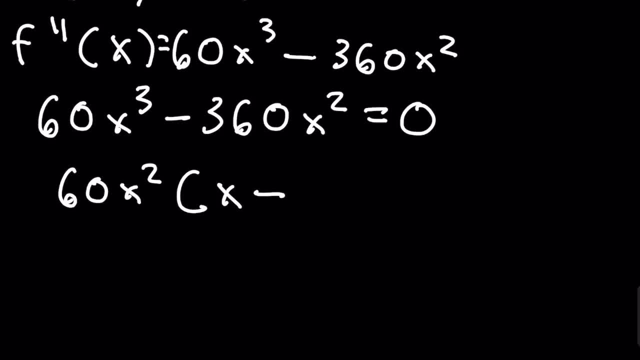 and then if we take out a 60x squared from 360x squared, we just get a six. So we have 60x squared multiplied by x minus six equals zero. So what values of x will make this zero? Well, if we plug in zero, zero squared is zero, and then 60 times zero is zero, So zero. 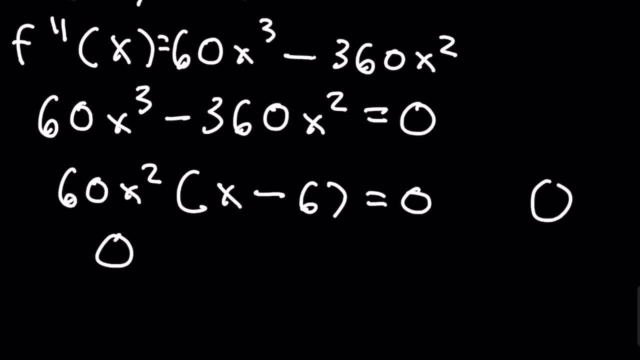 times a number is just zero. So zero is one of our numbers to get it to equal zero. But what else could do it? If we plug in a six right here, we'll get six minus six equals zero, And then 60 times. 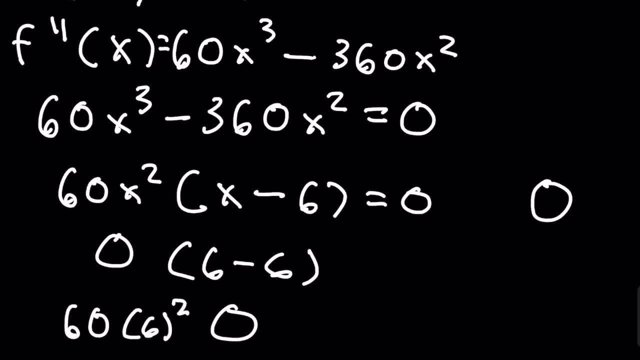 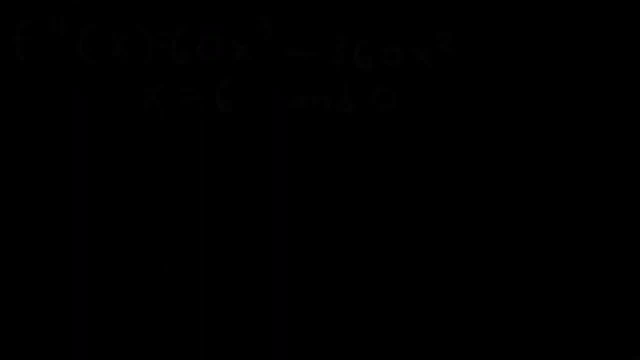 six squared is just going to be a positive number, and any number times zero is zero. So our two values that make our second derivative equal to zero are six and zero. So now that we got our two values when solving for zero, which in this case is six and zero, 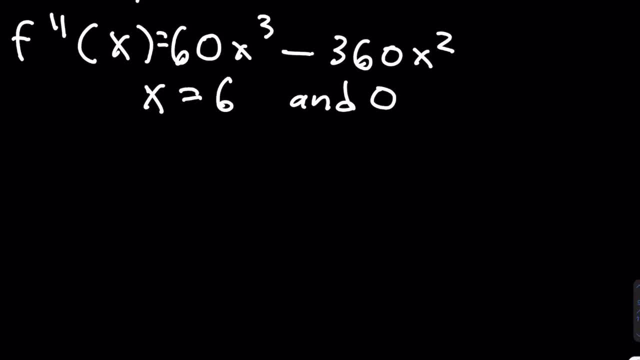 these are going to be our possible inflection points. So after we find these, what we're going to want to do is plot them on a number line. So let me plot six and zero on here. And so in order for something to be an inflection point, it must go from concave up to concave down. 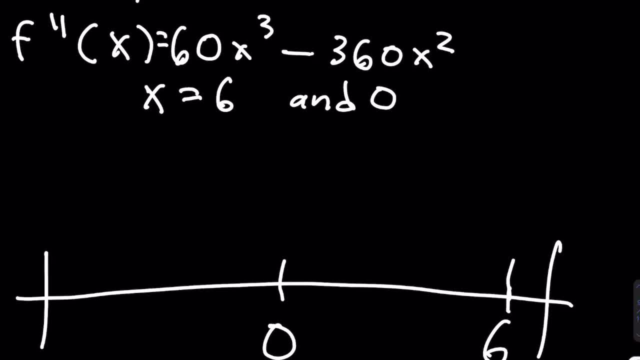 or concave up to concave down, So it can go either of those ways. So what we need to do is check whether the left side of our values versus the right side of our values it must switch Concave up to concave down or vice versa. So let's check the left side of zero first, And so 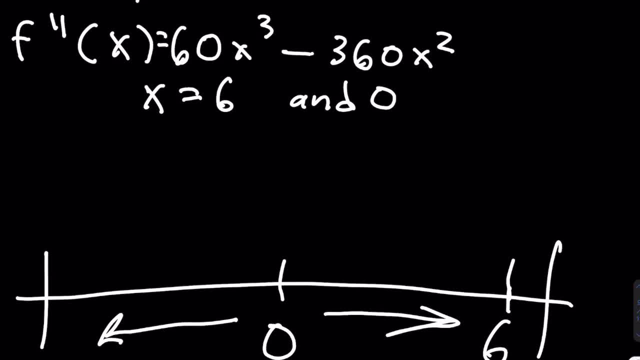 in order to determine whether it's concave up or concave down, we need to take a value that's less than it and plug it into our second derivative equation. So let's take the value minus one, since it's less than zero. So 60 times minus one cubed is just 60 times minus one minus 360 times minus. 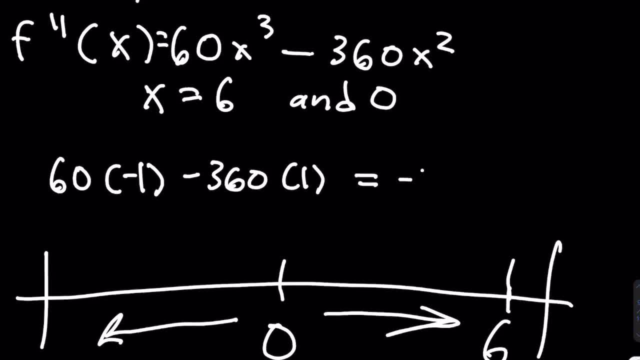 one squared is just one. So this is going to be equal to minus four 420.. So minus 420 is is less than zero. So that means this is going to be concave down. So now let's check the right side and determine whether or not it's concave up or concave down. So if we plug in a number, 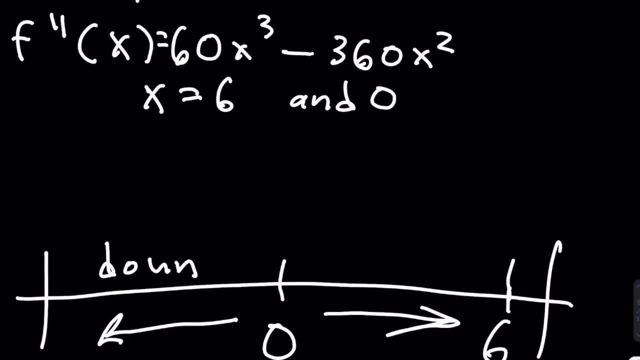 from zero to six, let's plug in one. So 60 times one cubed is just 60 times one, minus 360 times one squared, which is so that's one. And then 60 times minus 360 is going to be minus 300.. 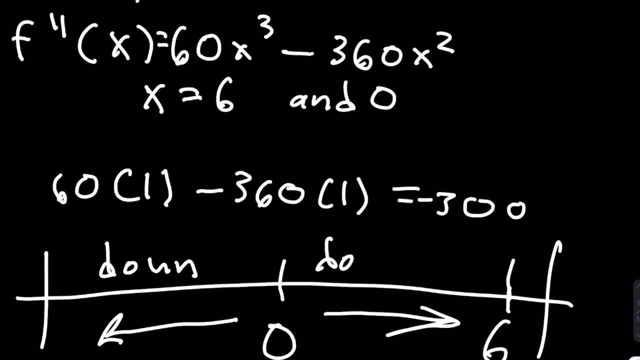 So this is also less than zero. So then this means that this is concave down. So that means, since zero is down to down, so concave down to concave down. that means that it's not going to be an inflection point, but we still can try six. So let's try the right side of six. Let's plug in. 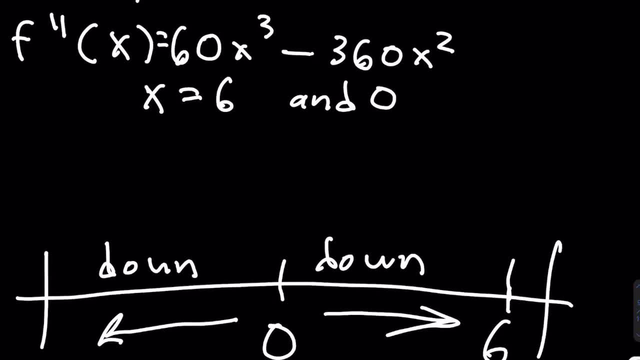 the value 10.. So if we plug in the value 10 to this, we're going to get 60 times 10 cubed, which is 60 times a thousand, minus 360 times 10 squared, which is a hundred. So this is going to be 60,000. 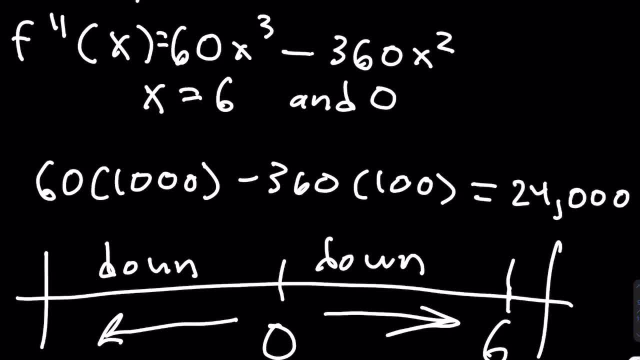 minus 30.. This is going to be 6,000, which is 24,000.. So 24,000 is greater than zero. So that means this is going to be concave up. So on the left side of six we're concave down, but on the right side 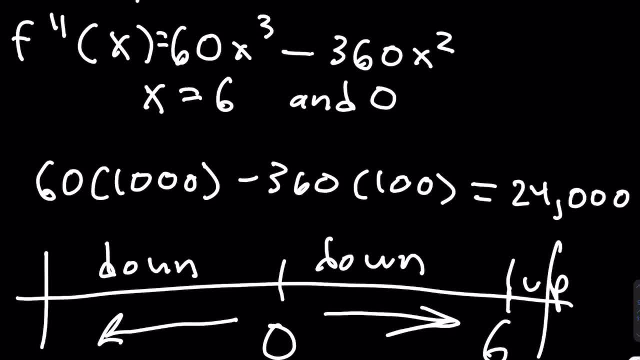 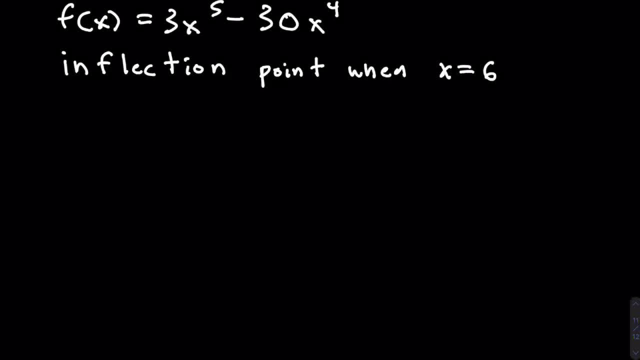 of six we're concave up. So because it switches from down to up, that means six is an inflection point, And so that's the only inflection point of our function. So now that we know we have an inflection point when X is equal to six, in order to find the X and Y point for the inflection, 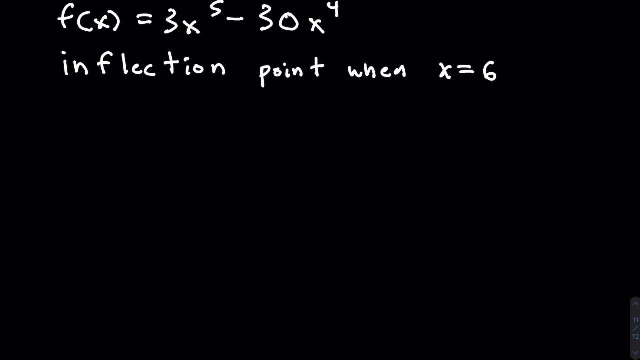 point, we need to plug six back into our original equation. So when we do that, we'll have three times six to the fifth, minus 30 times six to the fourth. So six to the fifth is 7,776, minus 30 times six to the fourth, which is 1,296.. So three times 7,796 is 23,328.. 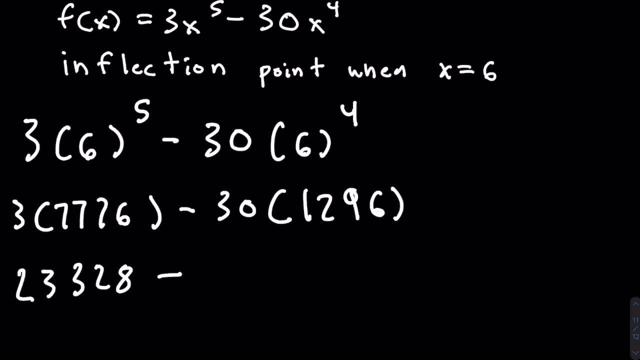 And then 30 times 1,296 is 38,880.. And so when we subtract these we'll get our Y value, which is negative 15,552.. So that means our point of inflection is at: X equals six, and then our Y is negative 15,552. 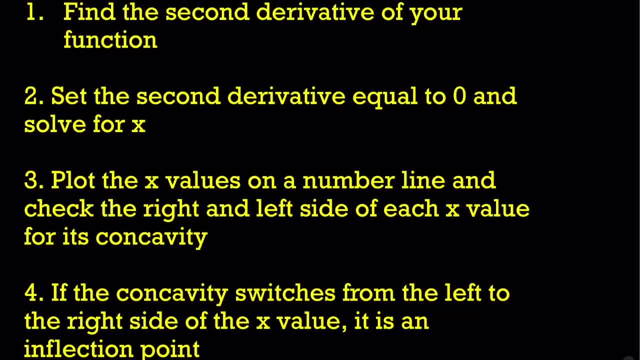 So let's review how to find an inflection point. The first step, what you're going to want to do is find the second derivative of your function, And after you find the second derivative of your function, you're going to set it equal to zero and then solve for X, And these X values are going. 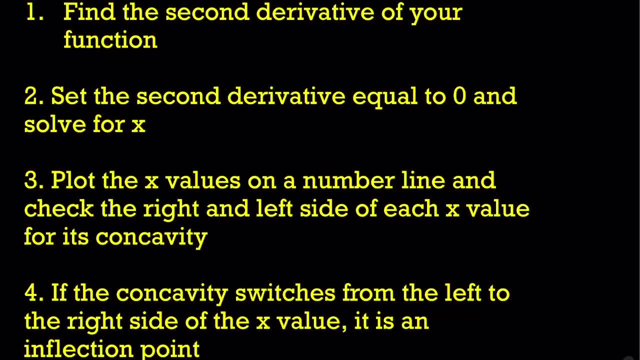 to be your possible inflection points And then, after you have these X values, you're going to plot these on a number line. And then, once you have them on the number line, you're going to check the right and left side of each of the X values to see each of their concavities And if 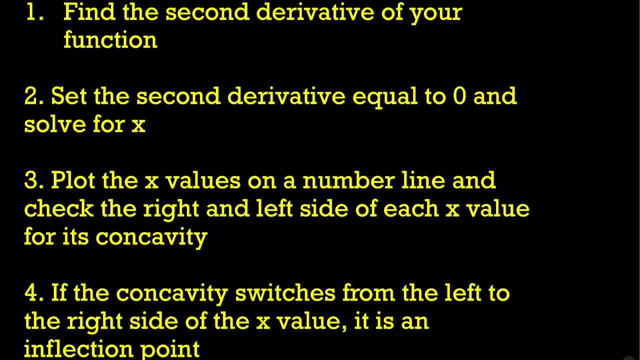 the left side concavity after it crosses the point and on the right side of the concavity and they swap. so if it goes from up to down or down to up after crossing the point, then you know it's an inflection point. But if it doesn't, you're going to have to do the same thing. You're going to 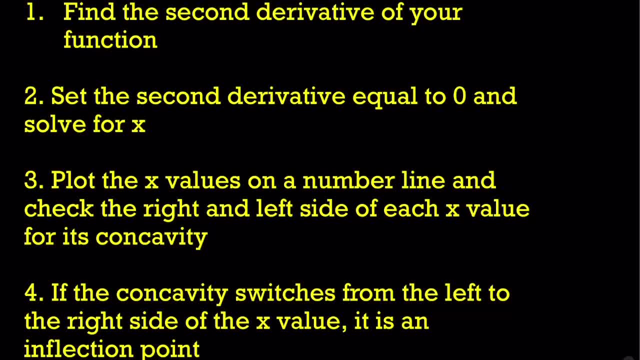 change. it just stays from like up to up or it goes from down to down, And that means it's not an inflection point. Thanks for watching today's video and subscribe for more math help.